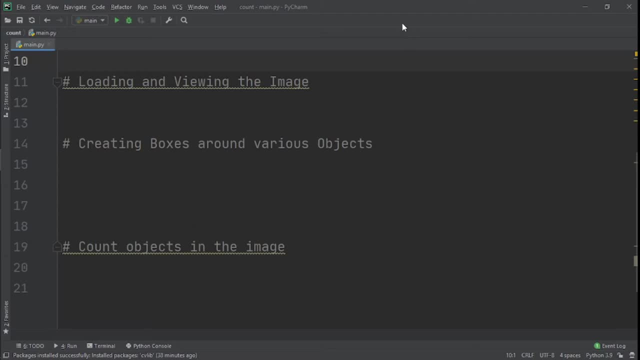 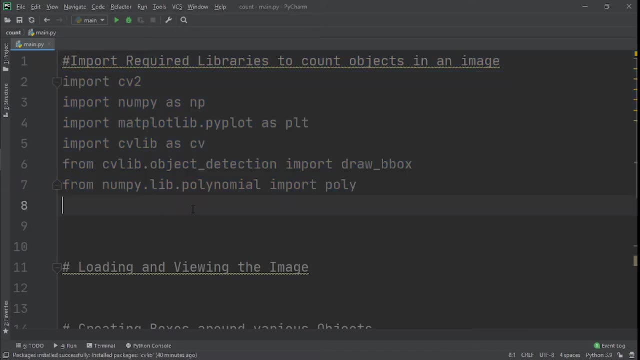 page and in that web page all you need to do is copy the command and you paste it in your terminal right here so you can see that it's going to power this whole project and it's going to power this whole project so you can see all the libraries right here. so the libraries we need, we need open. 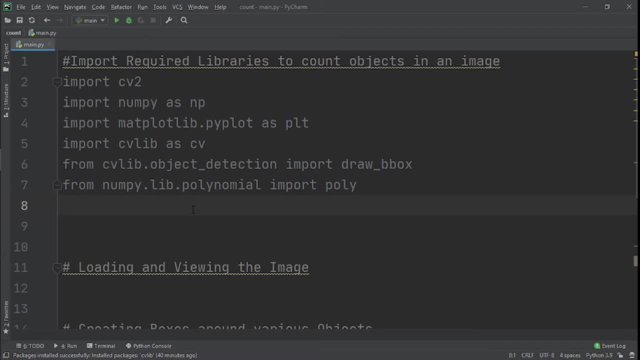 cv module. we also need numpy module, we also need matplotlib module and after that we also need cvlib module. we'll need also object detection and dropbox sub module of cvlib and also make use of the numpy polynomial module as well. so you can see all of them right here. i will leave in the 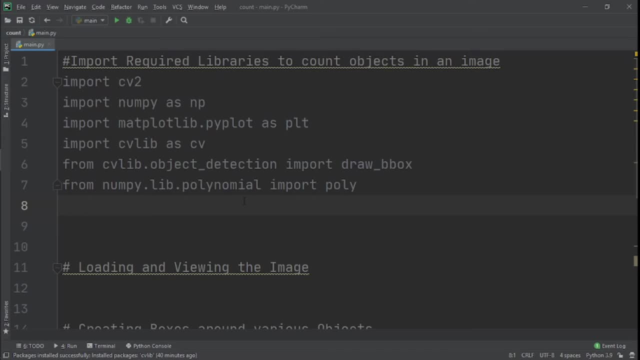 description guys, a starter file, and all you need to do is just get that starter file and you see all these modules. all the modules are in there and you can see all the modules are in there and already written down for you. so just to make it easy and speed up the process. now what we need to 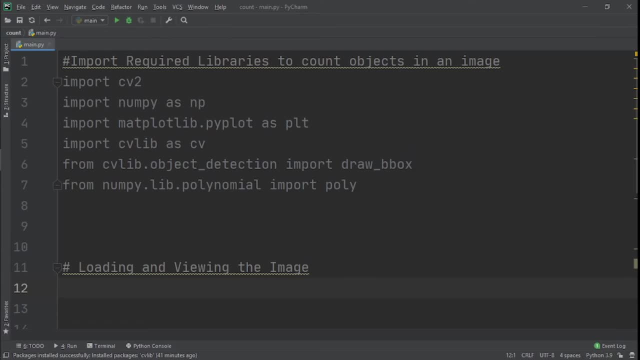 do is we need to actually load and view the image. so we're going to be loading and viewing the image and guys look to load an image. we need to make use of the intread function of the cvlib library and pass the name of the image as a parameter. so you need to make sure the image is stored in the 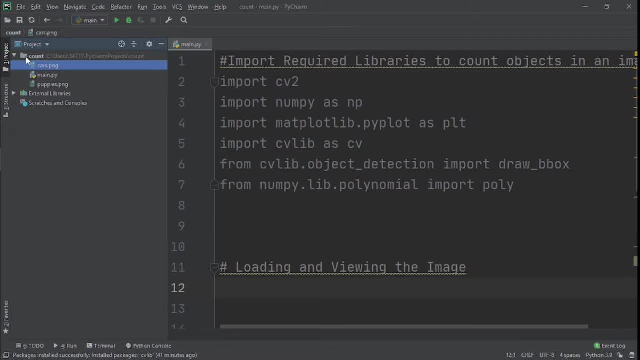 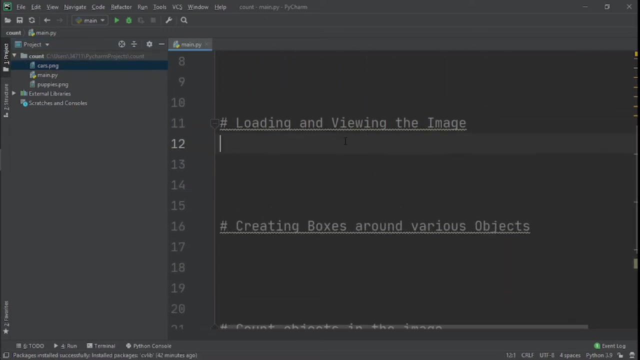 same directory as your code. now, look guys, you can see right here that i have a project called count and inside this count we have our mainpy and then we have the two images, cardspy and also poppiespy. so, look guys, this is how we're going to load and also view the image. 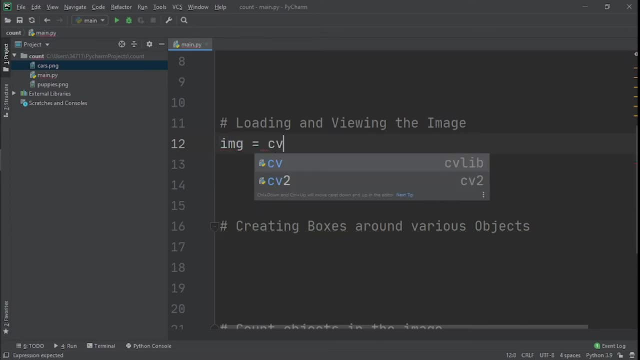 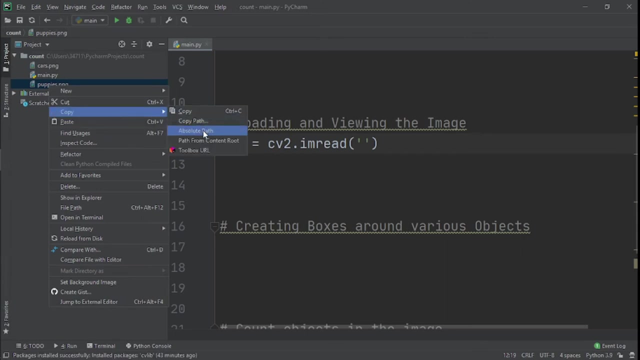 we'll say: image is equal to cv2, dot, imread. so this is what i mean by mread or imread, or yeah, whatever you prefer. and now we need to put the directory of our file. now, look guys, to get the directory of this image right here, this puppy's image, you right click and then you hover on copy and you click on absolute path. so 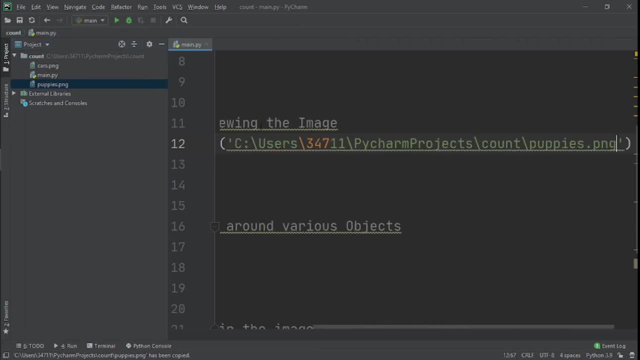 now, we've just copied the absolute path. we'll paste it right here. but what we need to do next is we need to change this right here to this. so just the other, this slash to the other kind of slash. so you do that for all of them and yeah, so that's all you need to do for the image. 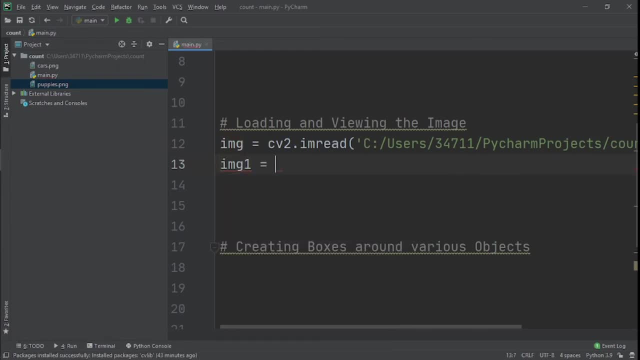 and after that we'll say: image one is equal to cv2 dot- cvt color. i will put as in a parameter the image and then we'll say cv2 dot- color in capital and we'll use this right here. so we use this, so we get it in the right color. 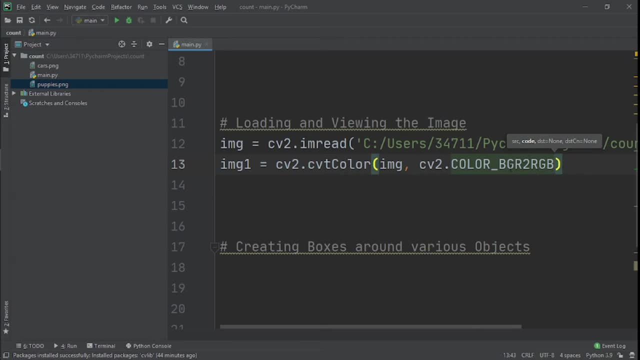 it chooses one of these colors right here, which is rgb and also bgr. now, after that, we'll say plt and small letters, we'll say plt. dot figure, i will say fig size, we'll make it 10, we'll make it 10 and 10.. 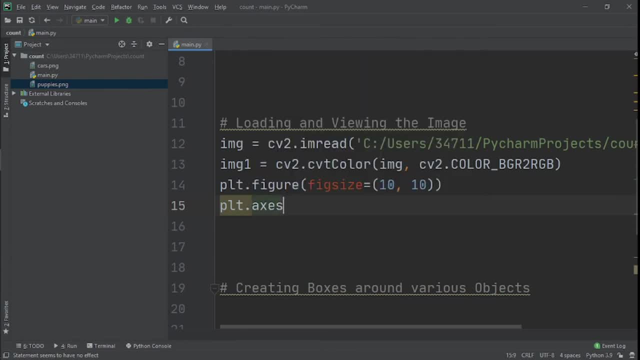 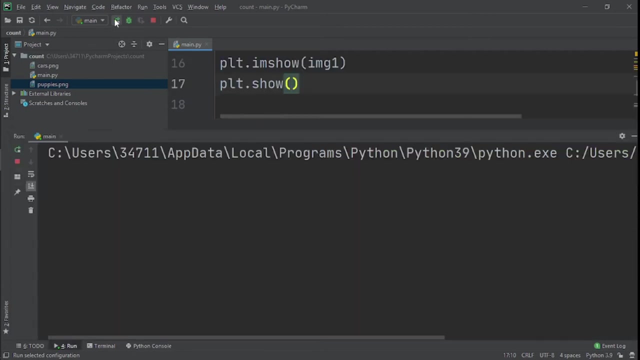 now we'll say plt dot axis, i'll set that to off. after that we'll say plt dot, i'm show, i'll say image, we'll put image one. now we just say plt dot show to actually show it to us. so if we run this, you can see it's loading, you can see the tensorflow and all that. 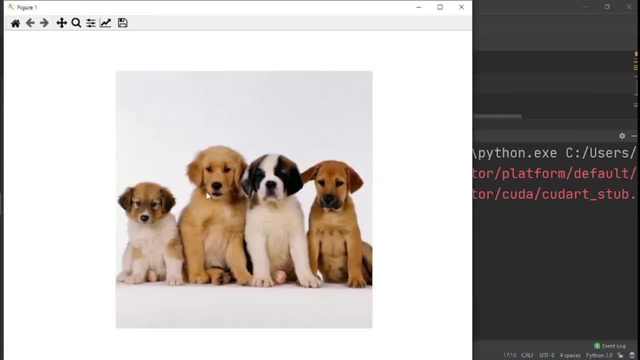 so after that we should actually see. now we can see the image. you see this cute puppies, yeah, my favorite is: you know what i like? all of that, like all of them. I don't really have a favorite here. they all look really cute. so now we can see. 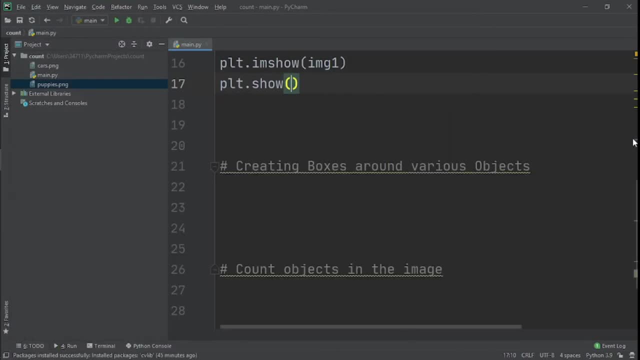 our image, but that's not the final project. so what we need to do next is we need to create the boxes around the various images, because we'll create the boxes and after that we'll just count the boxes. now, look guys, for us to create the boxes around the various objects. what we need to do is we need. 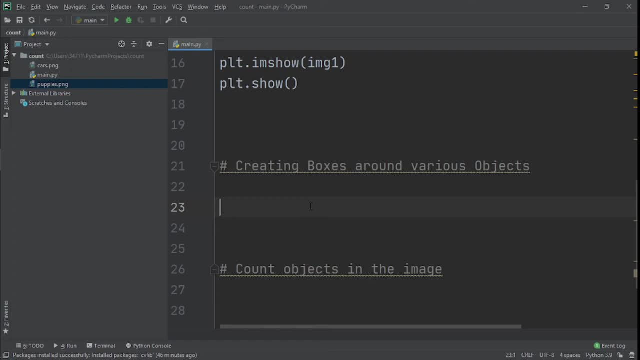 to firstly use the detect common object function and pass our image as the object for it. and while we're using this function, is that this function will return the box, the label and the count of the box to the generated object on our object detection, and after that we need to draw the 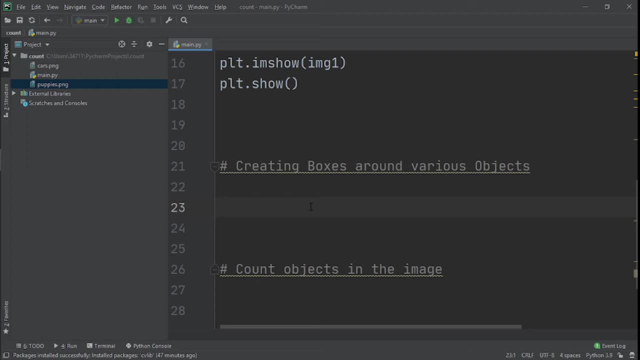 boxes. so we need to use the draw b box function and pass the output received by the various functions to this function. so hopefully you understand that. but I'll show you right now. what we do is: we say box and then we say label, then we say count, we set that equal to c. 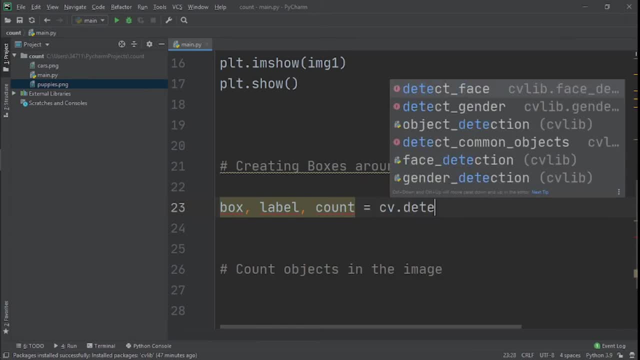 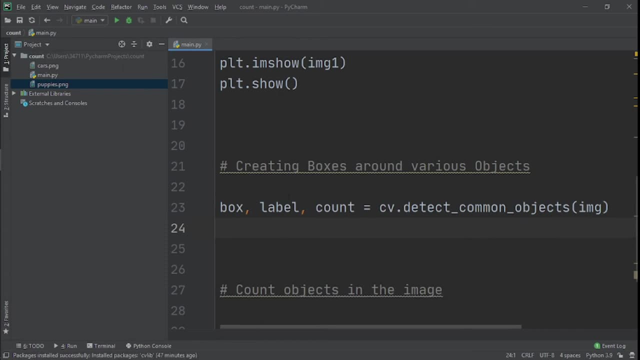 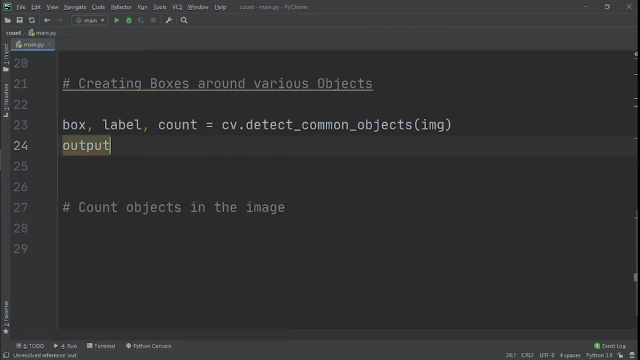 v dot detect common objects. I'll pass here our image and after we pass our image, we'll say: output is equal to draw b box. then we're passing the image, passing the box, passing the label and also count. now, look guys, what we need to do next is we need to display the output image and we do that with. 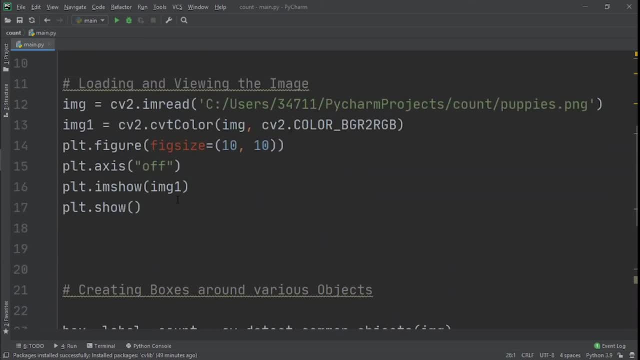 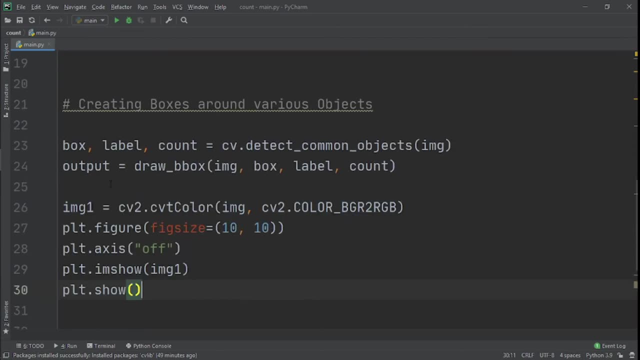 the amp show function again now, and how we do that is, we can just copy this right here. yeah, we just copy this right here, the one we use for image one. we paste it right here, but we'll pull output now and here, instead of image, we'll put output. 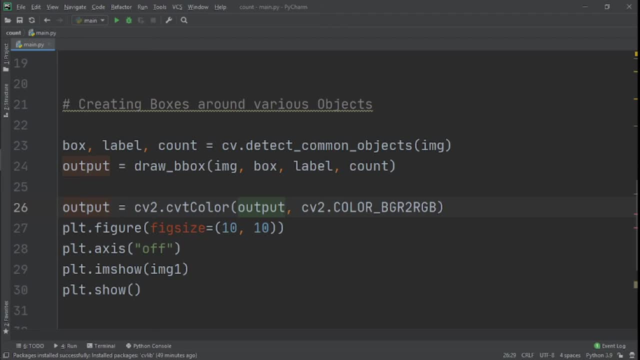 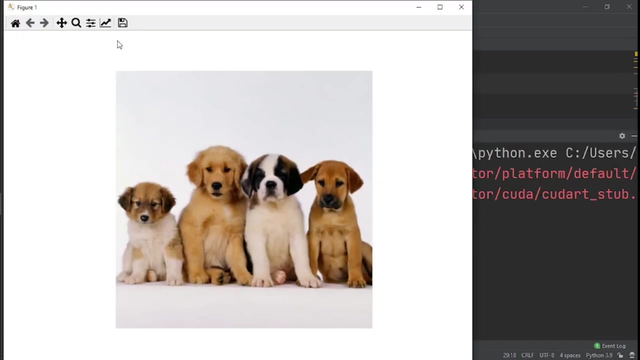 and here to put output instead of image one. so if we run it again, yeah, I'm going to cancel this. so we get the other one, because that's how my plot works. you can see now. we get them with the boxes around them and we have four boxes of these cute puppies. 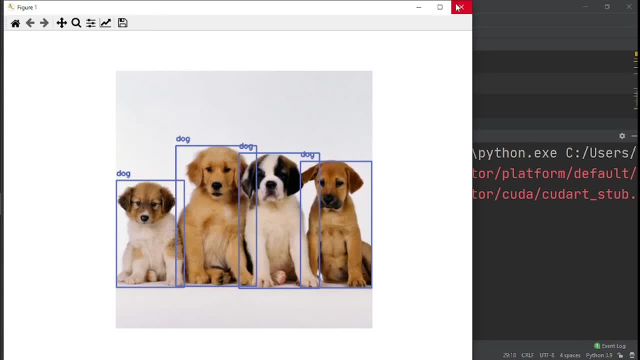 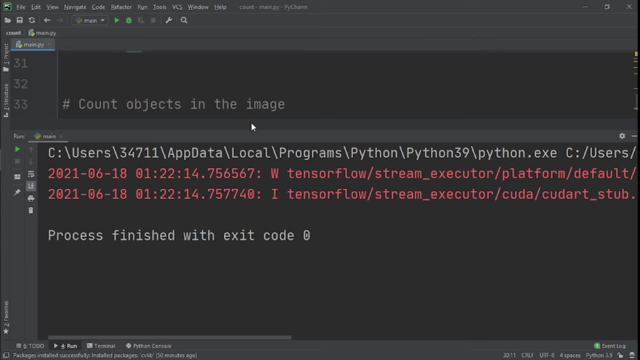 because there are four puppies there. so we see that it's working out well. finally, what we need to do is we need to just count them and we need to paste actually the number- I can see right here that we have the comment for that. we need to count the objects in the image.